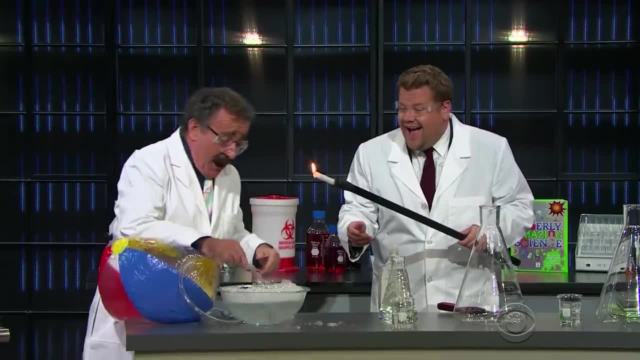 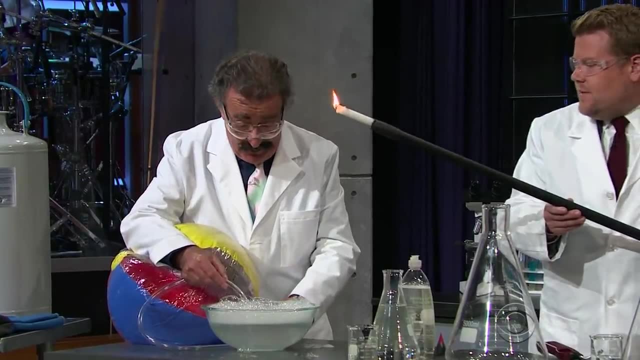 But that's in your hand. Actually, to tell you the truth, this experiment's a lot safer than the next one. Can I light one that's flying? Go on, give me a. Yeah, come on, Let's get a flyer up there. 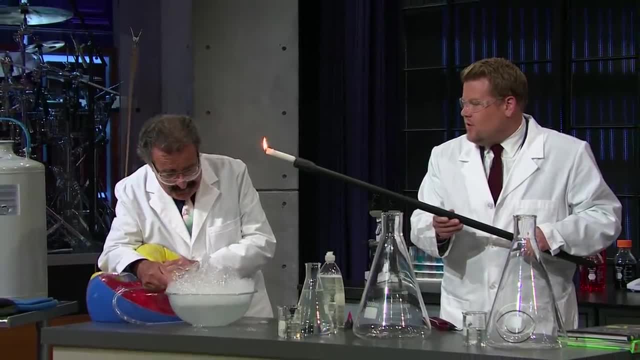 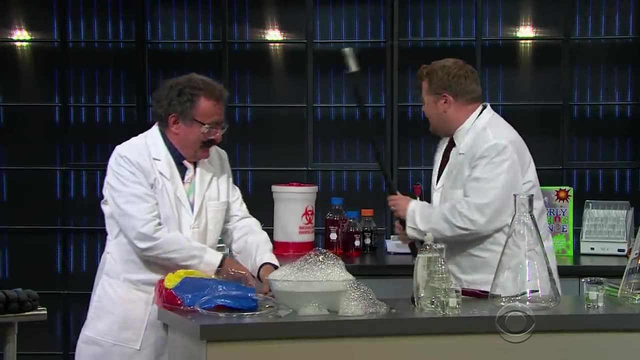 Rob, come on, here we go. Come on, Come on you, Come on you Go. James CHEERING- Oh it's beautiful. All right, so that's gas number one. Well, that's Your hand's all right. 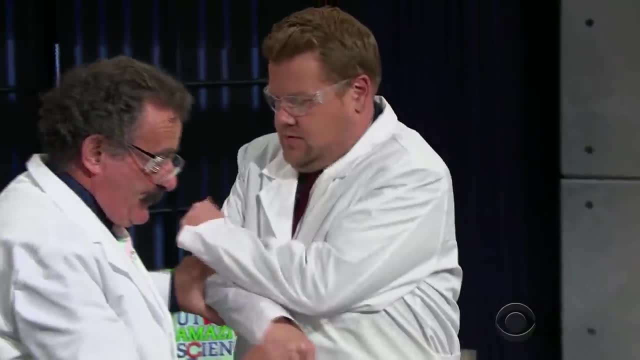 All right, rub them on me, Rub them on me, Go on, rub them on me. There you go. That's hydrogen. All right, that's hydrogen. What's next Tomorrow's fuel? OK, let me move this back a touch. There we go. 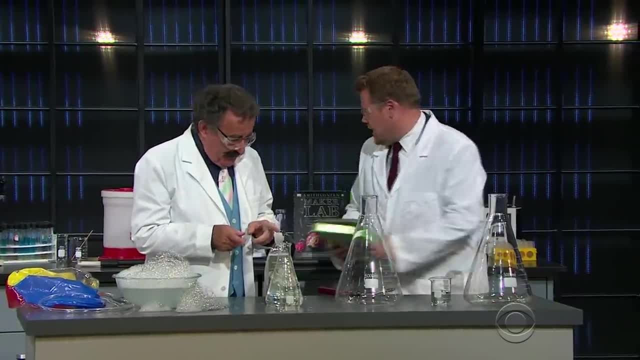 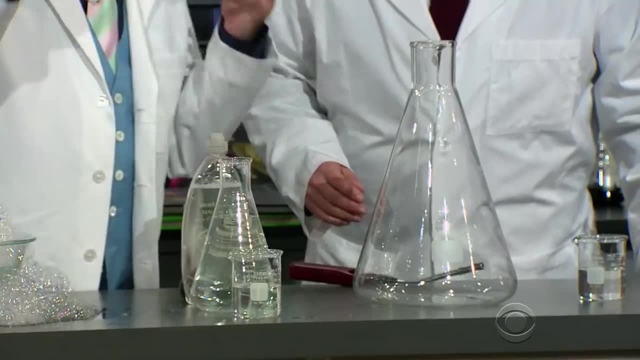 All right, that's tomorrow's fuel. What about this one? This is more dangerous, because this is What we're going to do- is to separate oxygen from what is a form of water- hydrogen peroxide, Yeah- which you'd normally use, perhaps, to dye your hair white. 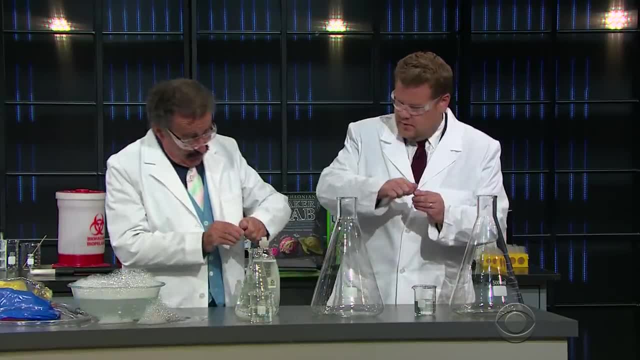 Now, what we're going to do is we're going to make a soapy solution with this coloured dye. So you're going to use red, OK, And how much of this do I put in? Well, put in the whole lot. 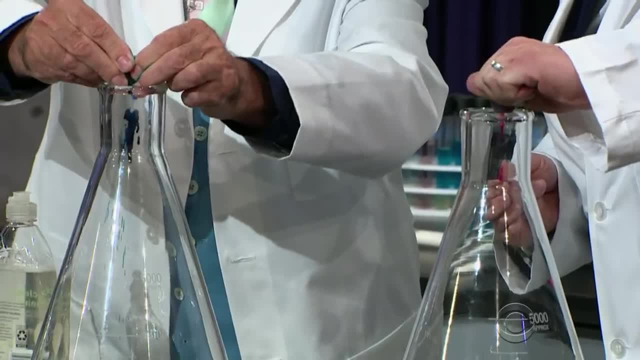 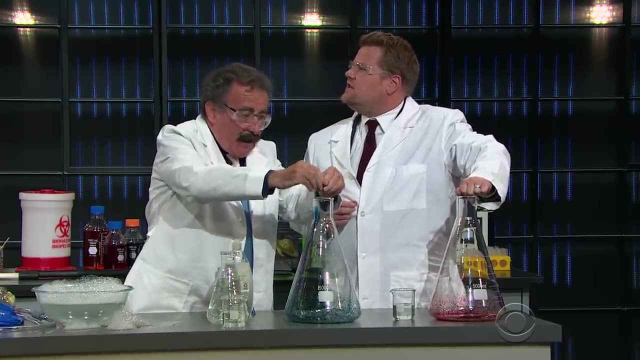 It'll take a while to do it, Because we need to make a nice soapy solution. A soapy solution, That's a good name for a band- Oh well, Reggie Watts and soapy solution. There we go. Now we'll put some nice soapy water in here. 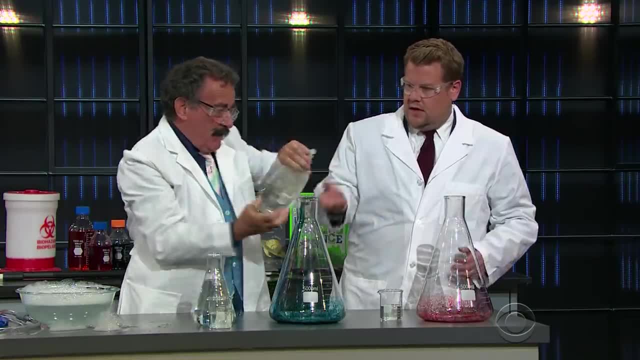 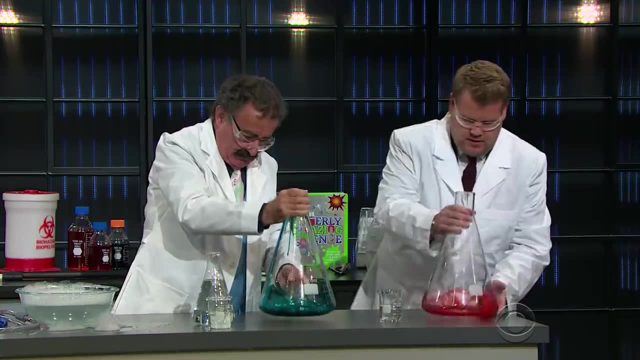 OK, All right, that's great, And make sure you get plenty in. I'm going to do the same in there. OK, Two, three, OK, All right, Now mess it up. Mix up this bad boy Now. 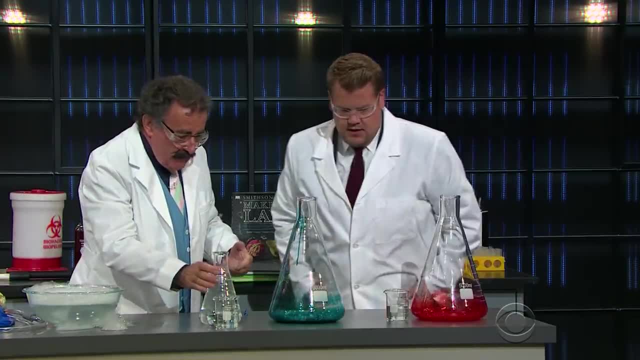 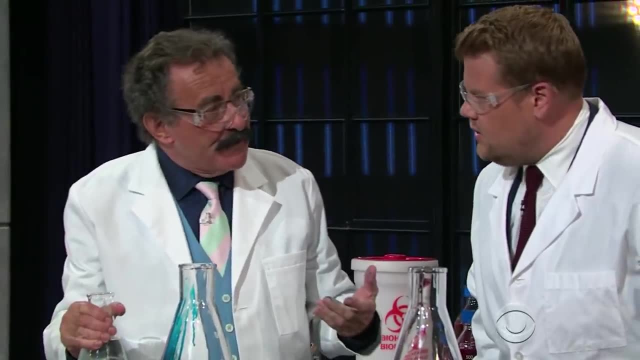 All right, OK, Now I'm not going to let you touch this, because it's just a Very wise, very wise. I should warn you that in the laboratory, I'm one of the clumsiest individuals, OK, And most of my experiments actually fail. 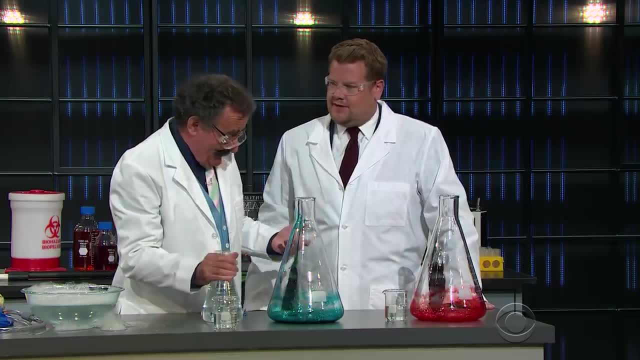 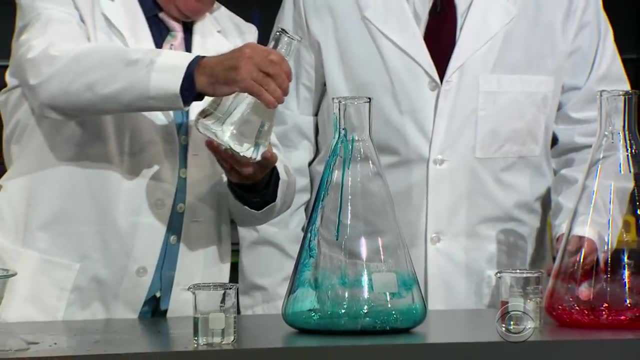 Oh, So Well, how wonderful that we flew you out here to do this. So I would suggest you just be careful, OK, and stand back when I tell you: All right, So we're going to pour this in, Right? 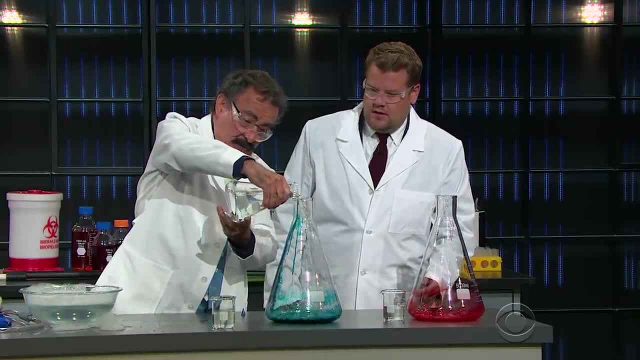 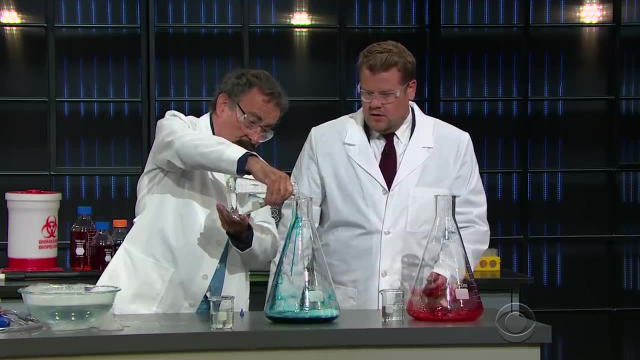 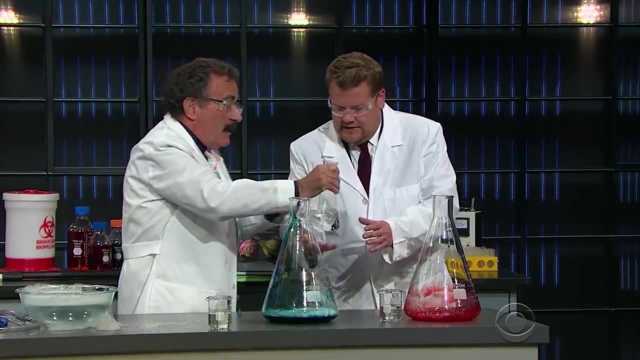 I'm going to pour half of it in: OK, My slask. So half of that goes in A little bit more. OK, Share and share. like you know, I pour this in here, but you're going to mix that around right. 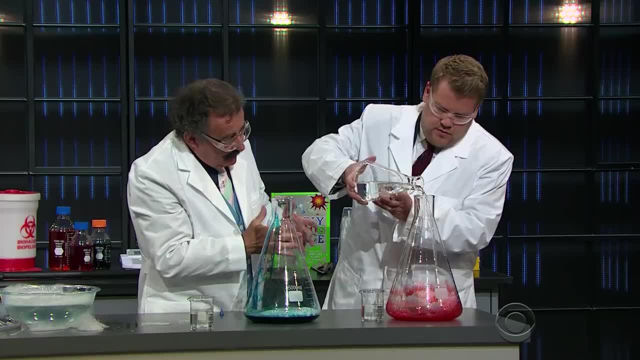 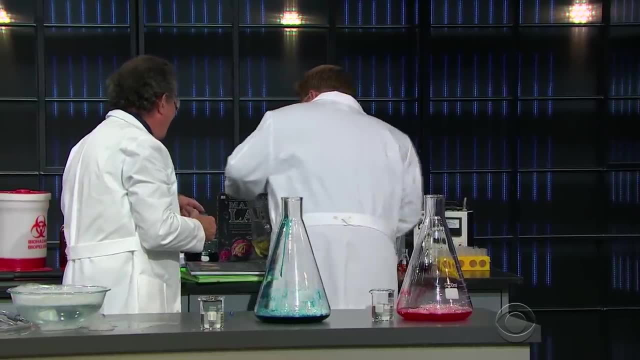 OK, I'm not going to. Don't worry, I'm not, Because your fingers will come off. Are you serious? I'm serious. OK, Now My turn. OK, It's all right, I've got it. So now we're going to. 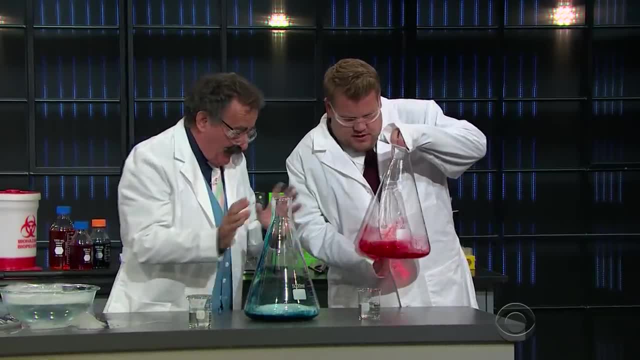 We're going to stir this around, Right? No, you don't need to stir it around, actually, It's all right. It's fine, That's all right. That's stirred. OK, that's mixed. I wouldn't touch it if I were you. 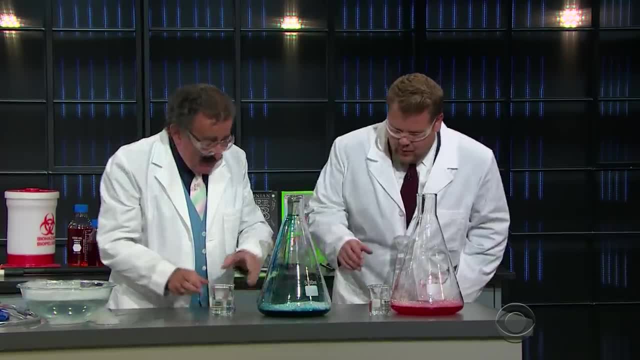 Now look, All right. And now what's this? What's going on here? That's That's. Shouldn't I have gloves on or something? What's going on? You should have gloves on Right. OK, go on. 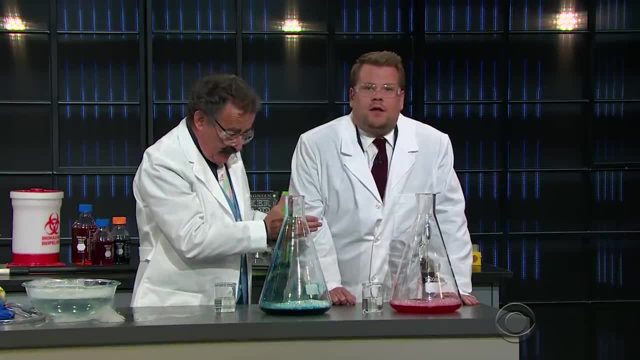 If we were doing this in the laboratory, we'd also have a shield here and a shield here. So we'll just keep your fingers crossed, OK, And we're going to Now. we're going to pour this in. I'll keep my fingers crossed if I've got fingers. 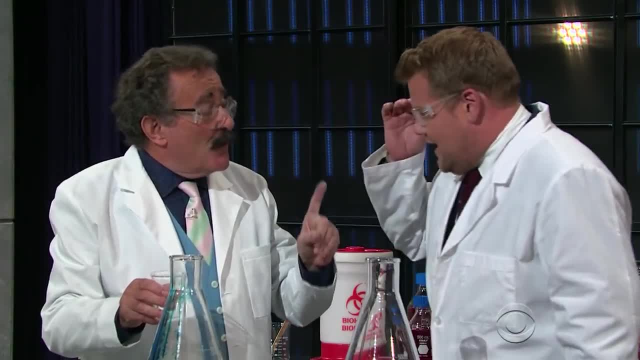 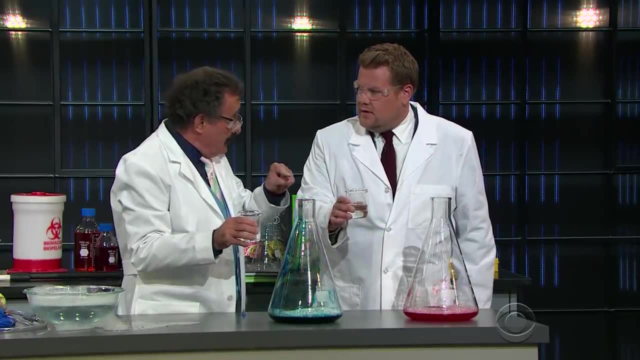 All right. yes, Games pay attention. I'm paying attention. Yes, OK, We're going to do this simultaneously. OK, So we're going to count to three. Yeah, All right, And on the third beat, we pour this in and we retire. 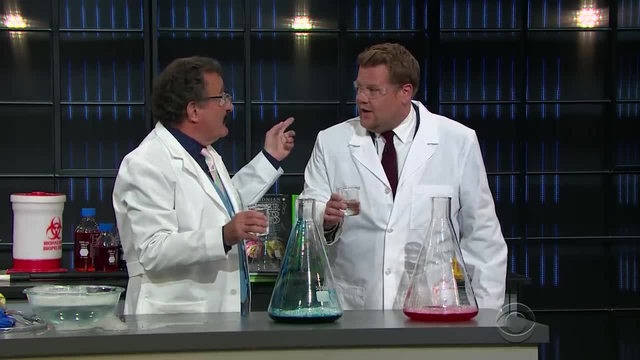 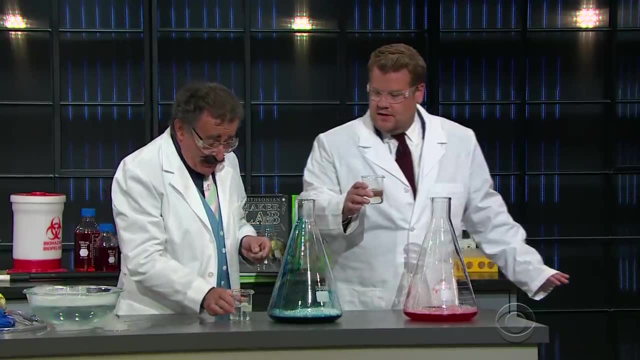 We get out of the way, We'll go behind Retire as in die or I'm not joking, OK, I'm dead serious. So we run away. Yeah, we run away. OK, Let's go for it. Three, two, one and run. 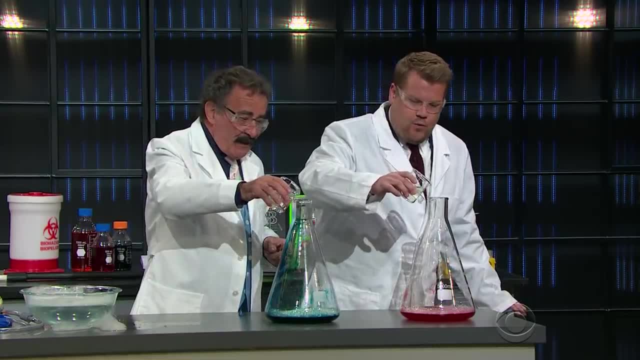 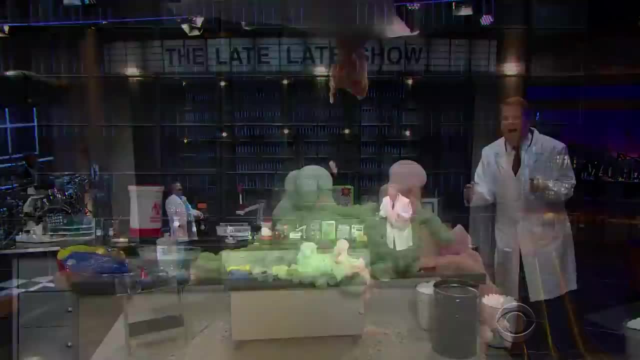 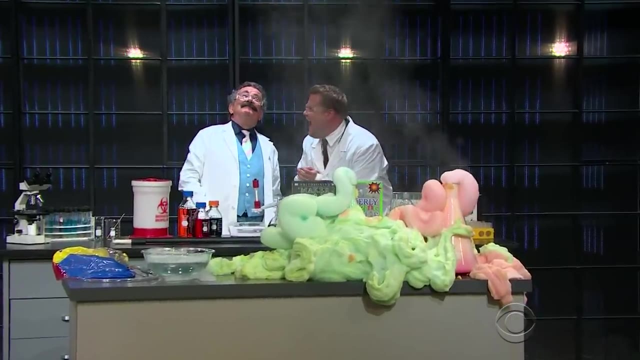 Three, two, one, or one, two, three, One, two, three, One, two, three. OK ready. One, two, three, Go, Go, Go, Oh ****, Oh ****, Oh, my word. 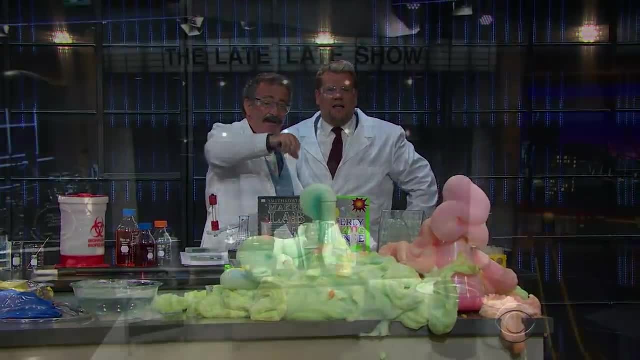 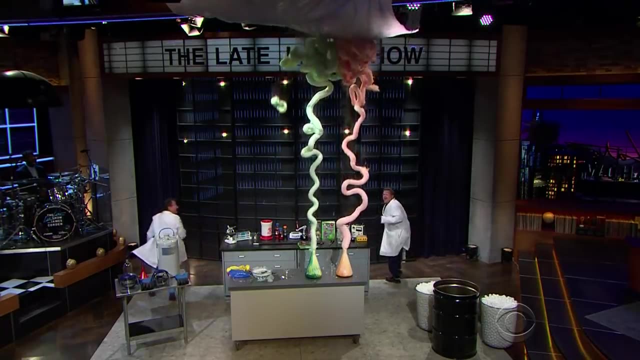 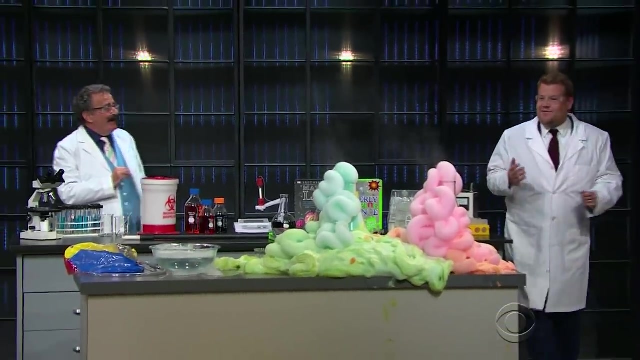 That's amazing. See how hot it is. You see the steam coming off. It wasn't quite a simultaneous orgasm, was it? It wasn't a simultaneous orgasm, but it was very much like my sex life with my wife. I did it. 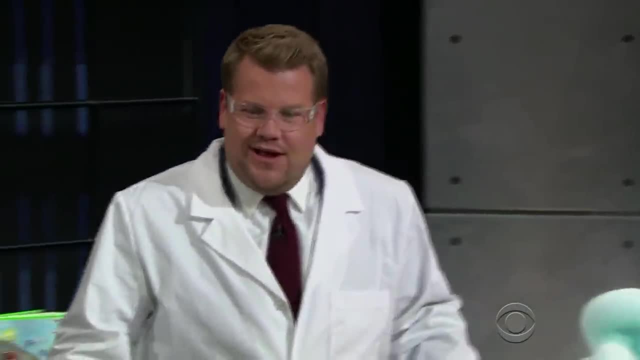 I ran away and let her just do whatever she needs to do, All right. So what's next? It's a dangerous experiment. What's next? This is dangerous. That wasn't dangerous. You told me I was going to lose my fingers. 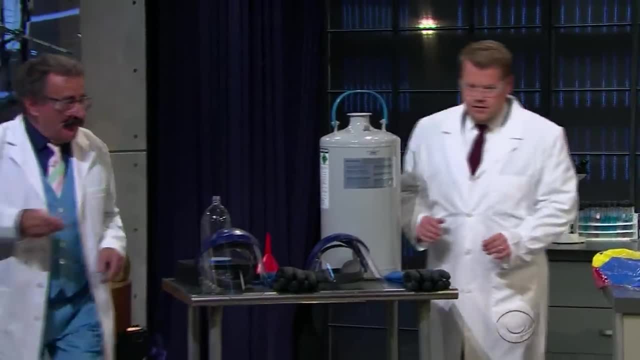 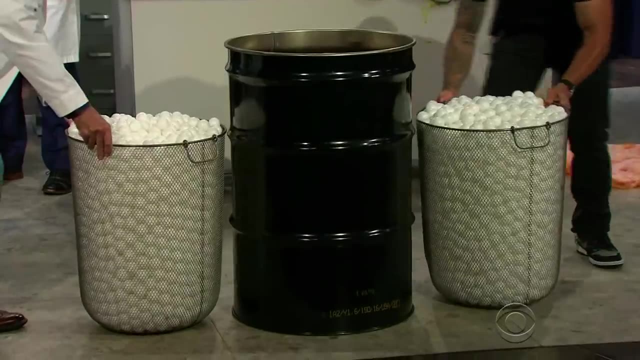 Right, What's this now? So what we're going to do is to put some. Do we need these on? I don't touch 4,000 table tennis balls and How are you getting through customs with all those? The person who's really 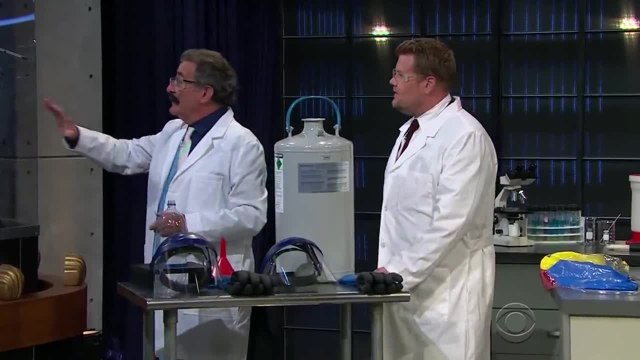 The person who's really at risk is Reggie, who I think probably ought to leave. because you're closest. We're going to be out of the way. Just step back. Well, what about the rest of the band? You don't care about them. 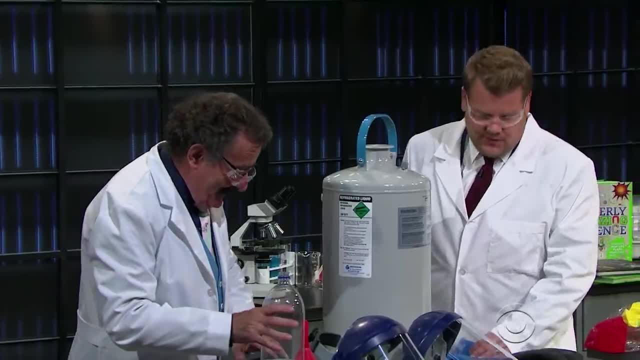 What are you saying? I mean, Hagar is literally half a centimetre away. All right, so what do we need? Do we need gloves on for this? We're going to put gloves on. Gloves on, Thank goodness. I really feel like I'm working in a lab. 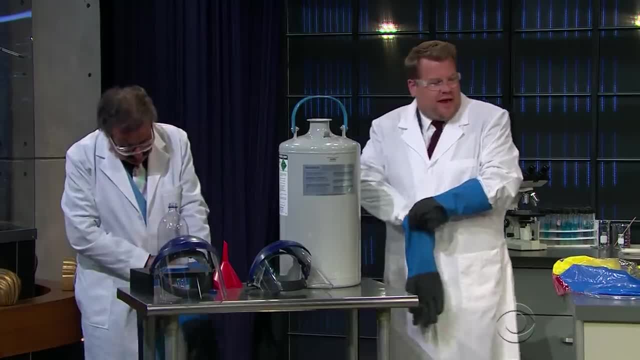 And what we've got in here. Now I can go home to my wife and be like, sorry, I'm late. Liquid nitrogen, Liquid nitrogen, Liquid nitrogen- Holy, That's the real deal. right, That's Which is cold. 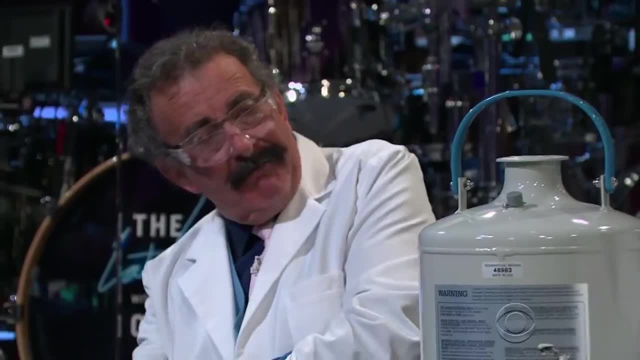 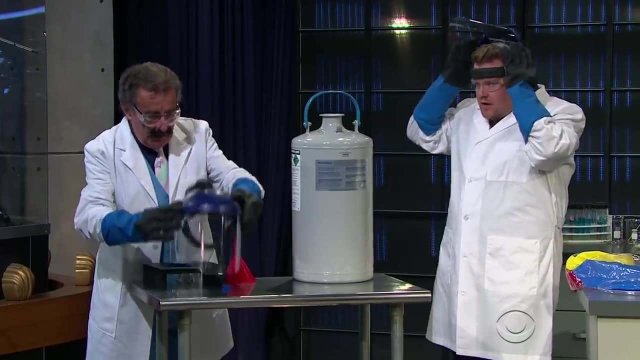 That's serious stuff. So it's about About 300.. Minus 320 degrees Fahrenheit. OK, About minus 196 degrees Celsius. So it's very, very cold. OK, And Tell me when to go so I can go. 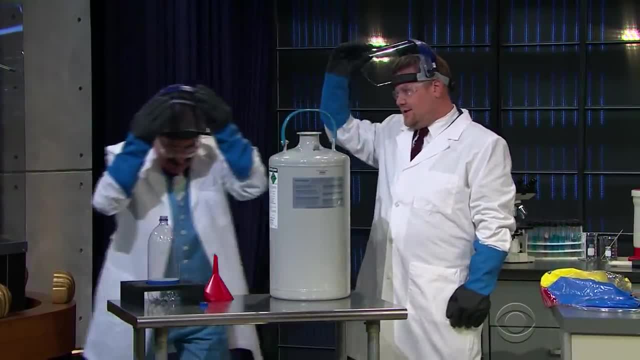 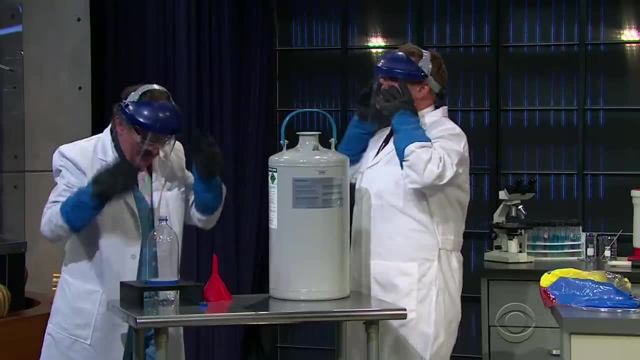 So when this warms up, When this liquid warms up, All right, When this liquid warms up and becomes a gas, it expands about 700 times. Oh yeah, this bad boy's going down Now. Now I need you to be really steady with this. 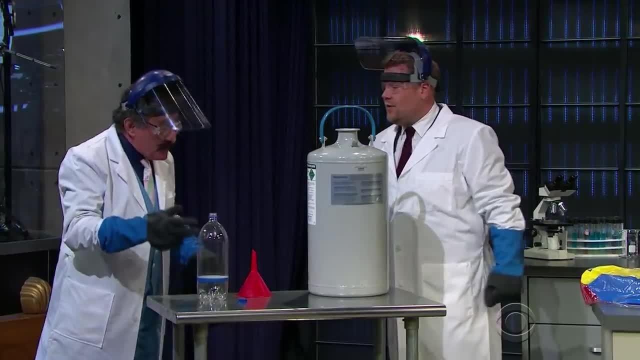 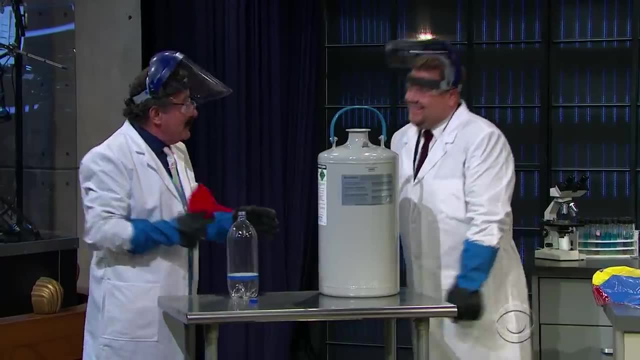 OK, Because I don't want this spilled over. Steady, Eddie they call me. You don't want it on the new suit. No, it's my genitals I'm worried about. I don't want. I mean, there's been a lot of genitals on this programme. 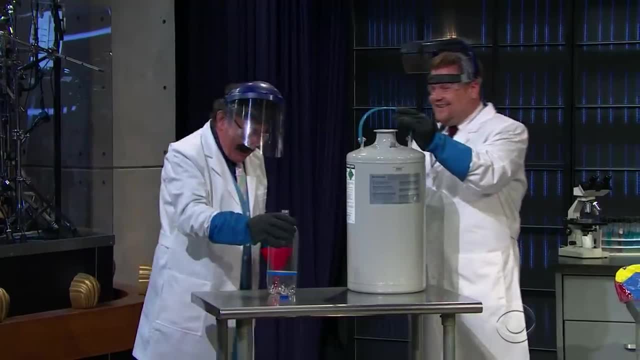 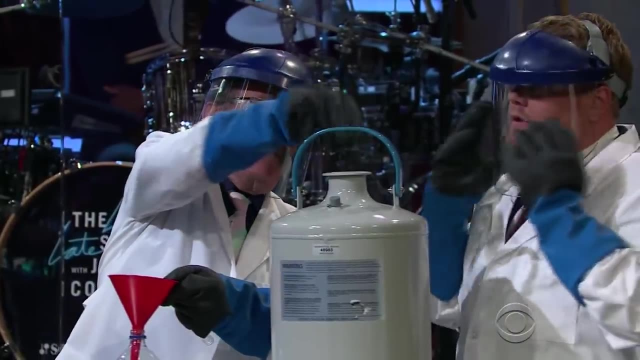 OK. yes, It's pretty disgusting. All right Now. all right, Visors, down Right. OK, So I'm going to fill the bottle up to the blue line. I want you to take the stopper out. That's it. 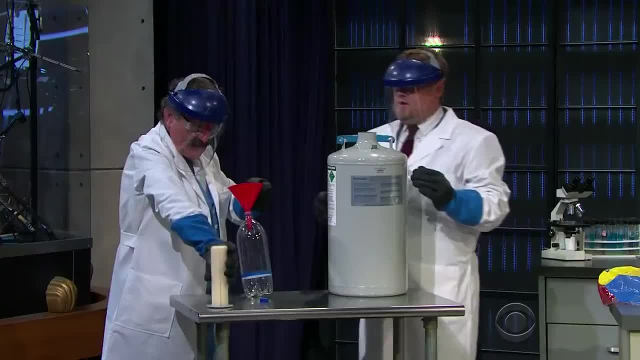 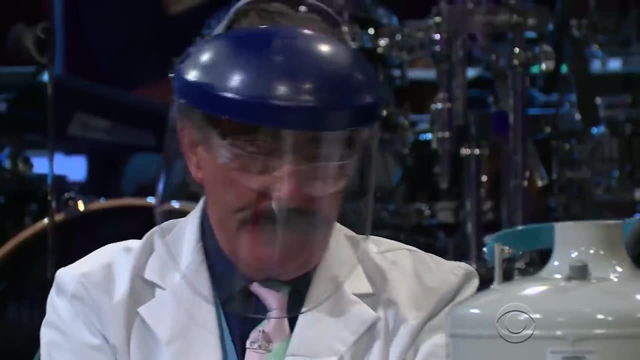 Oh, I already feel like I'm in science. OK, All right. In fact, let's put that down there Right Now, Pour this in there Pretty rapidly, but not so it overflows. Just up to here, Up to the blue line. 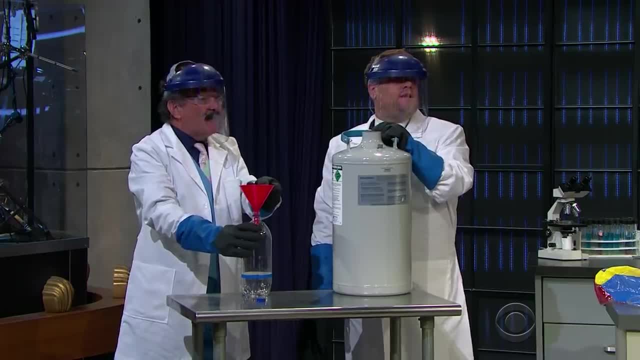 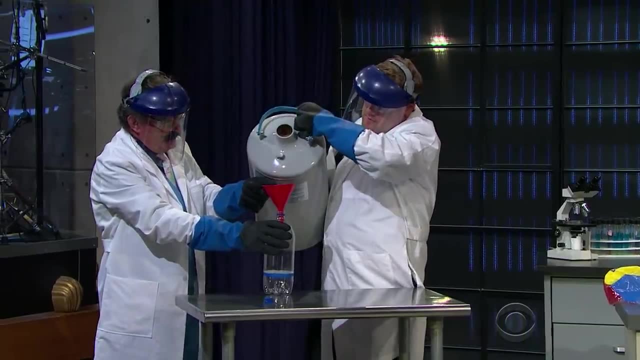 Why have we got such a huge thing of this? Why didn't we just get a smaller? That's to That's to protect you? What? All right, OK, here we go. Are you ready? It's coming in, Keep going.